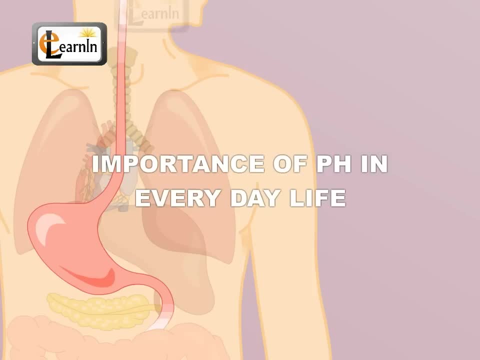 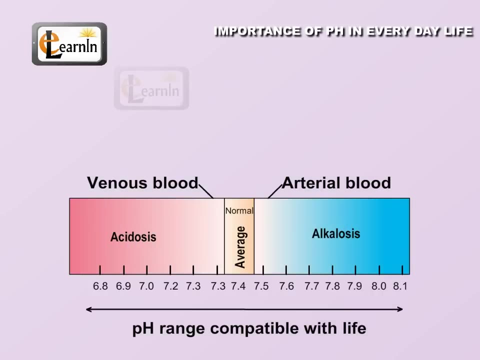 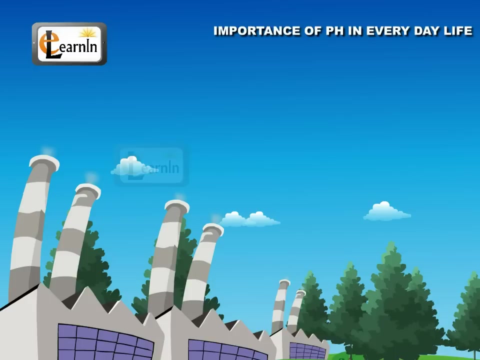 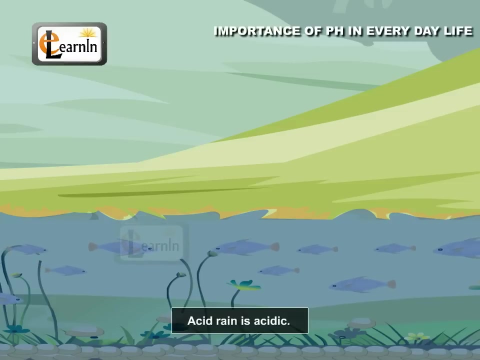 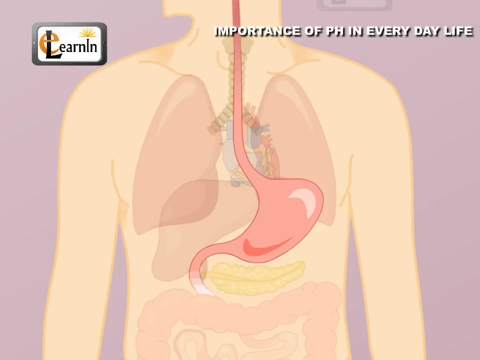 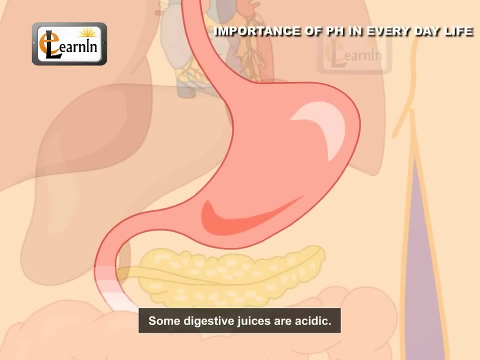 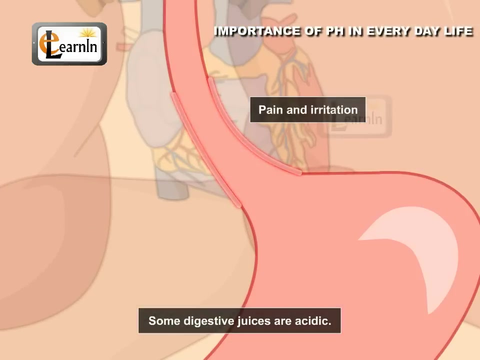 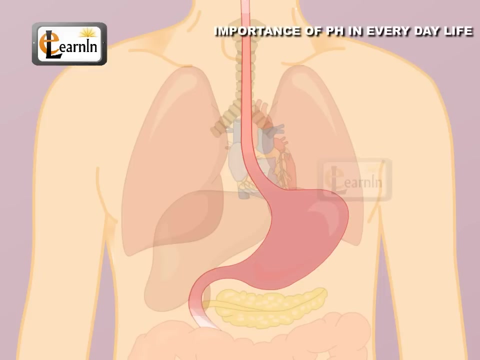 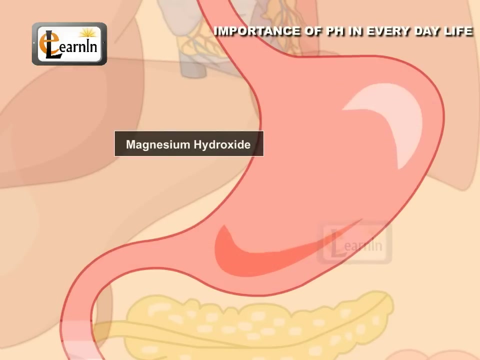 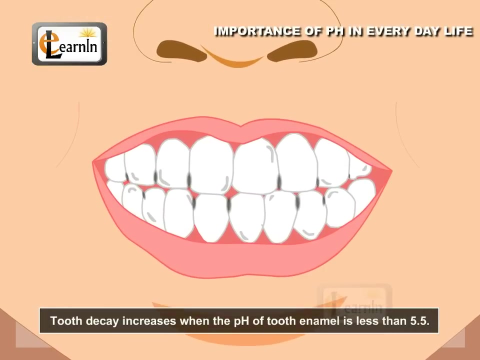 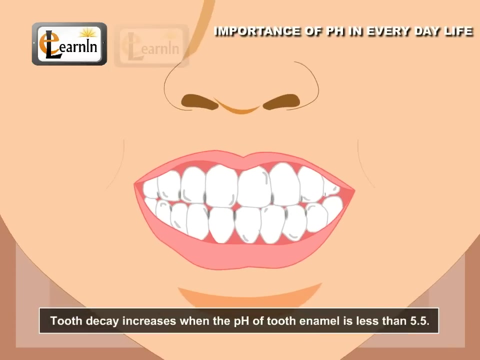 Importance of pH in everyday life Living organisms can survive only in a narrow range of pH change. The human body works within the pH range of 7.0 to 7.8. When the pH of rainwater is less than 5.6, it is called acid rain. When acid rain flows into the rivers, it lowers the pH of the river water, and the survival of aquatic life in such rivers becomes difficult. Plants require a specific pH range for their healthy growth. In terms of humans, it's very interesting to note that the stomach of a human body produces hydrochloric acid. It helps in the digestion of food without harming the stomach. During indigestion, the stomach produces too much acid and this causes pain and irritation. To get rid of this pain, people use bases called antacids. These antacids neutralize the excess acid. Magnesium hydroxide, which is also called milk of magnesia, a mild base, is often used for this purpose. Tooth decay starts when the pH of the mouth is lower than 5.5. Tooth enamel, made up of calcium phosphate, is the hardest substance in the body. It does not dissolve in water, but is corroded when the pH of the mouth is below 5.5. 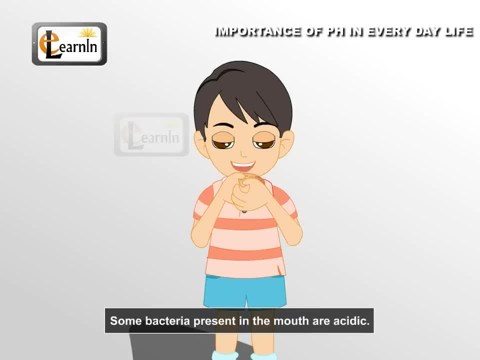 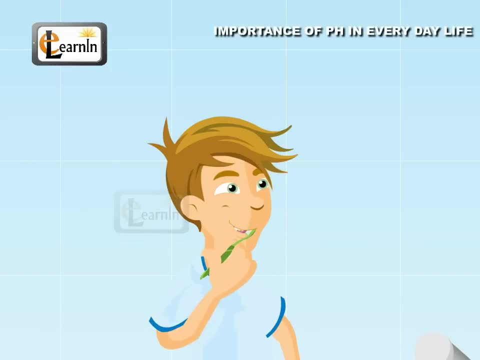 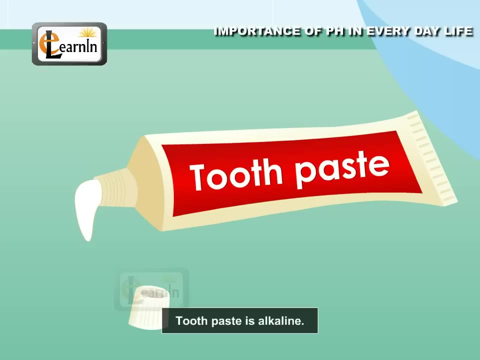 Bacteria present in the mouth produce acids by degradation of sugar and food particles remaining in the mouth after eating. The best way to prevent this is to clean the mouth after eating food. Using toothpaste, which are generally basic, for cleaning the teeth can neutralize the excess acid and prevent tooth decay. 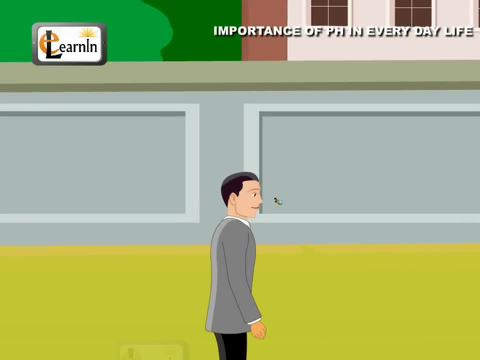 In the outside world, there are many other places that the human body encounters acid. For example, bee stings leave an acid that causes 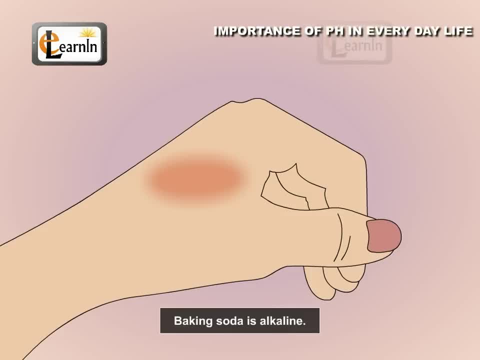 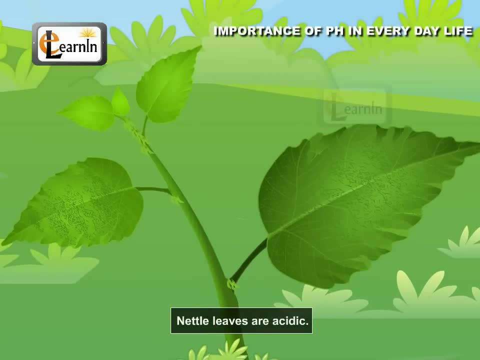 and irritation. Use of a mild base like baking soda on the stung area gives relief. Stinging hair of nettle leaves inject methanoic acid causing burning 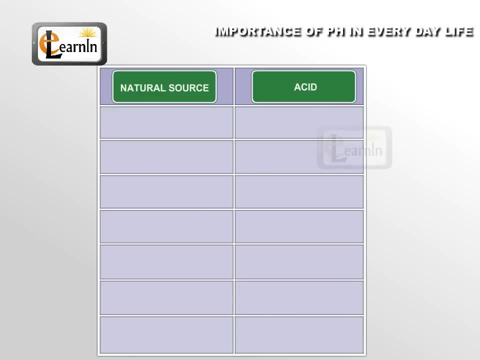 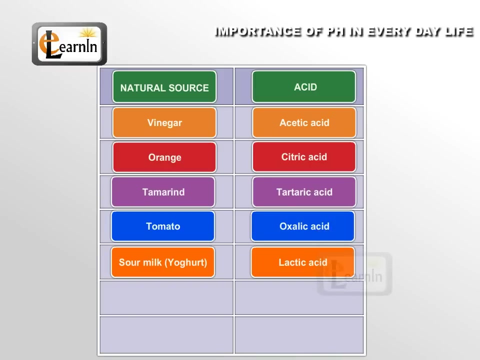 pain. Some more of the naturally occurring acids are vinegar which is acetic acid, orange which is citric acid, tamarind which is tartanic acid, tomato which is oxalic acid, sour milk or curd which is lactic acid, lemon which is also citric acid, ant sting which is methanoic acid, and